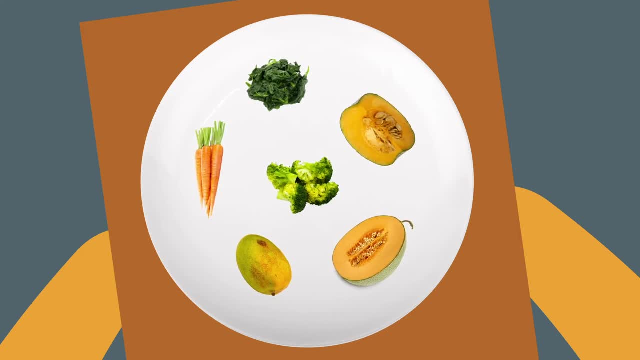 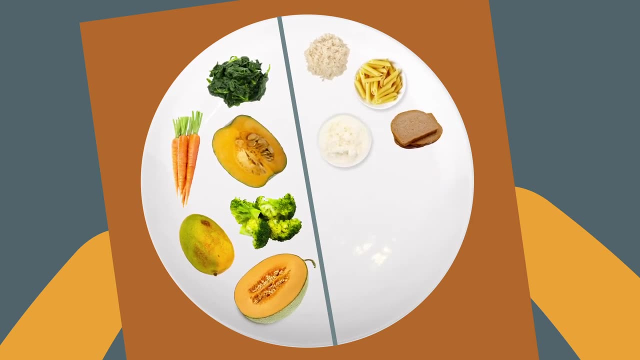 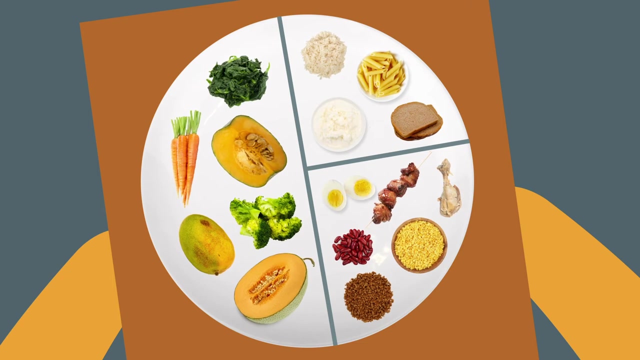 are good for your baby's health, So try to eat plenty of them. Also include some starchy foods like rice, pasta, bread and mille-mille, And don't forget protein-rich foods like eggs, meat, chicken, beans, soya or lentils. I know some of these healthy foods may not be appealing right now. 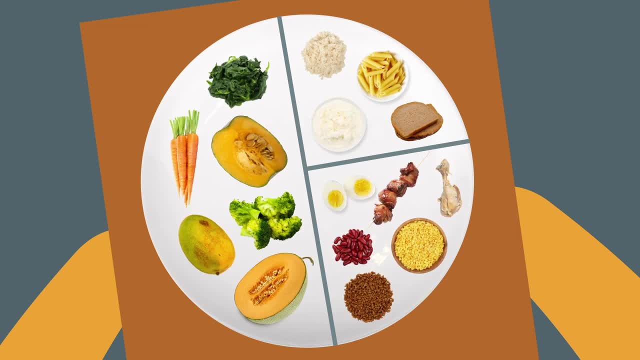 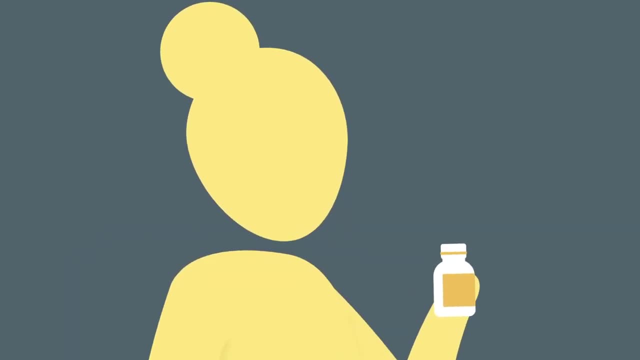 So do your best. Fatty, fried and salty foods do not have the nutrients that you and your baby need. So if I do all that, do I still have a baby? I still need to take the supplements I got from the clinic. Yes, Your body is working extra hard to grow your baby. 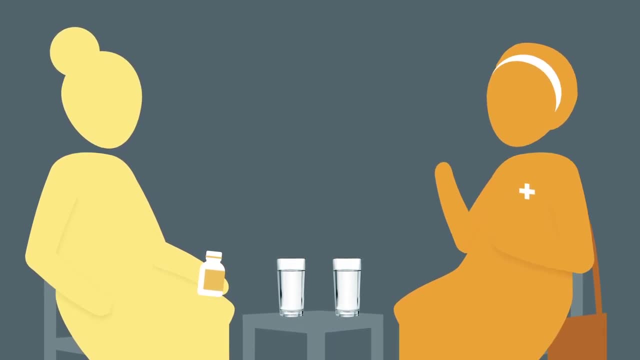 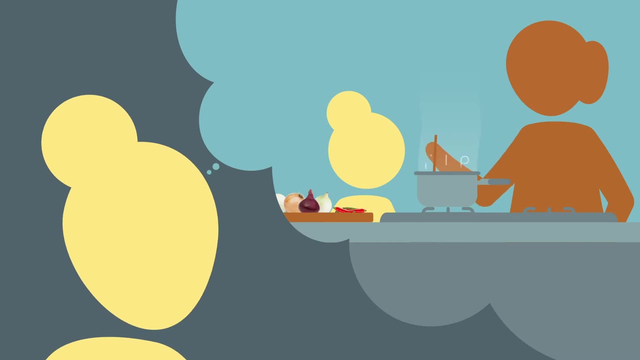 And the supplements ensure your baby has everything she needs. Okay, I can do this. I'm just sad that I can't make my special mincemeat fat cook anymore. Ever since I was a girl, I loved making fat cook with my go-go. 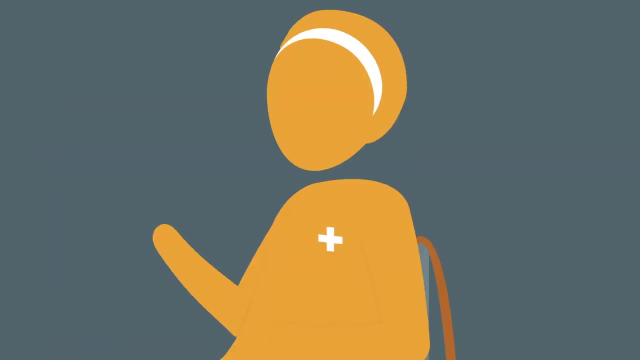 I was even hoping I could start my own business and sell them. You will be able to do that again soon, But in the meantime, why don't you try using new ingredients? You've always been creative in the kitchen. Just make sure to start by washing your hands with soap and clean water. 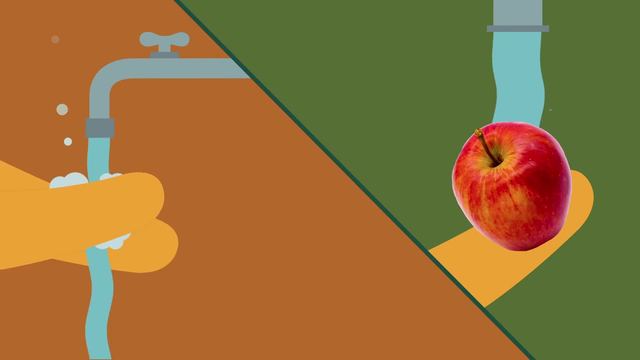 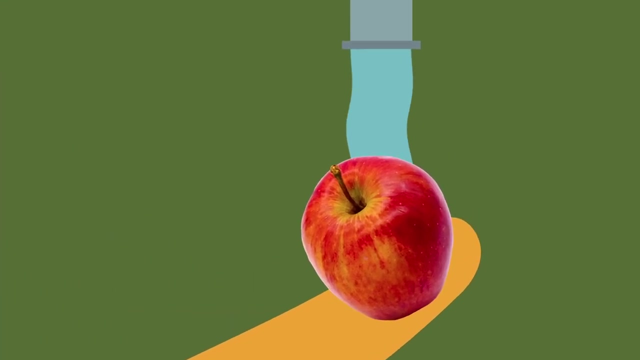 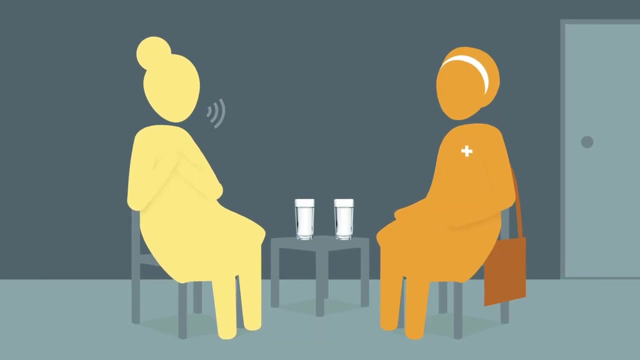 Wash raw fruits and vegetables in clean water before eating them. Cook meat, eggs and fish until they are well done. This prevents you from getting sick with bacteria or worms that will take away the nutrients you and your baby need. Thank you, Nomsa. This will be a good challenge for me. 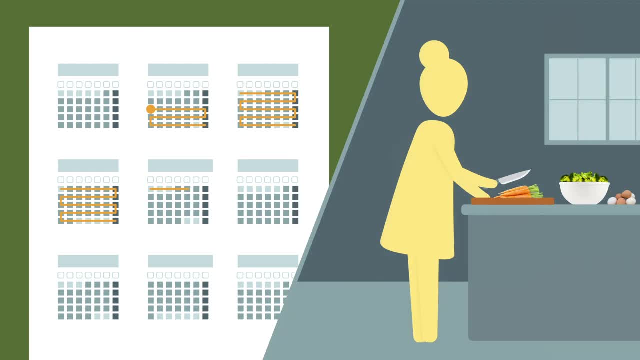 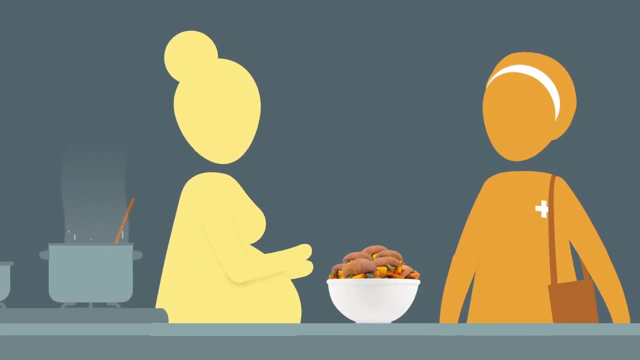 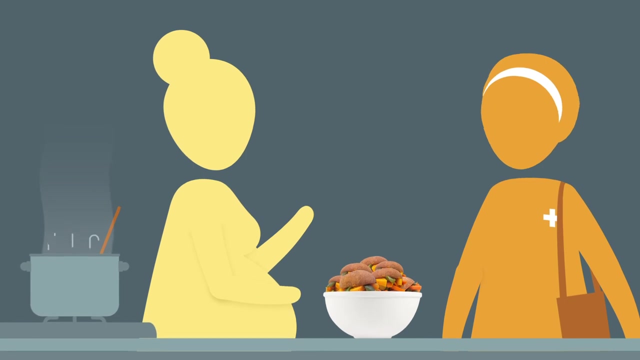 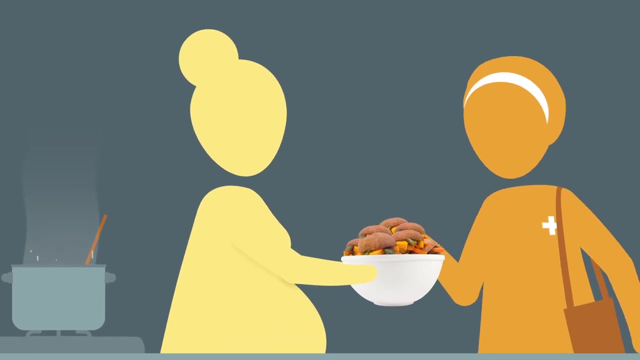 Thank you for your support and regular visits. I've been creating new recipes using the healthy food we talked about. They are even better than the mincemeat. I even have orders from neighbors who want to buy them. Try this. Mmm, this is delicious. 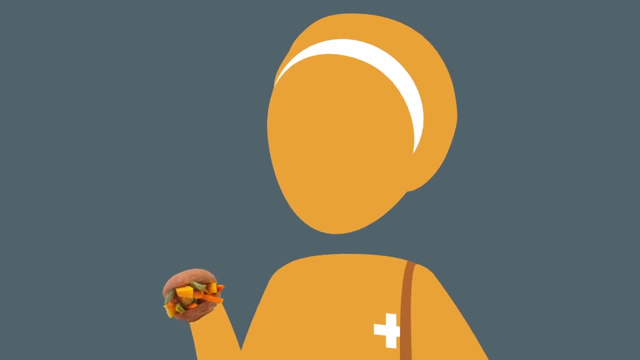 Your baby is lucky to have such a healthy and creative mama.